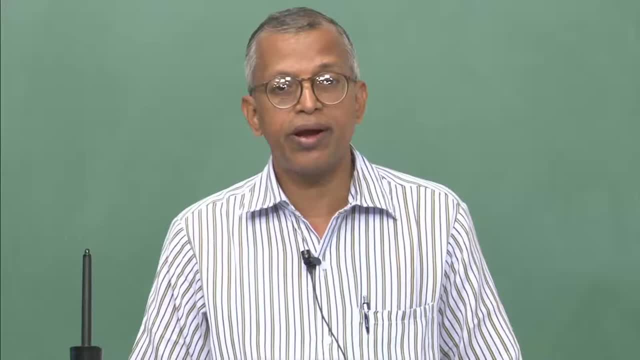 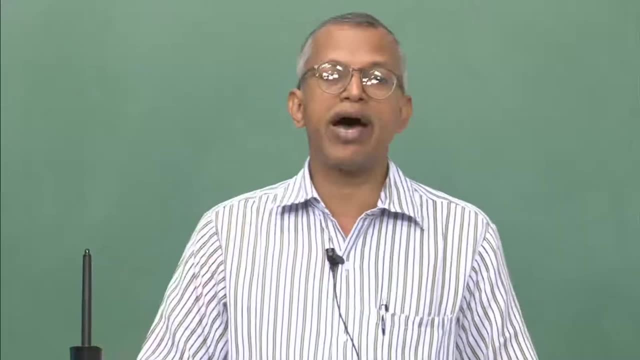 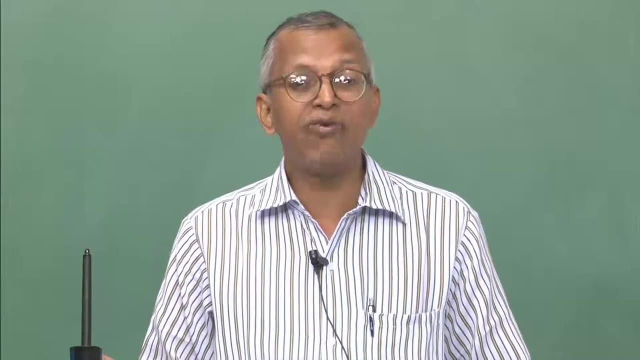 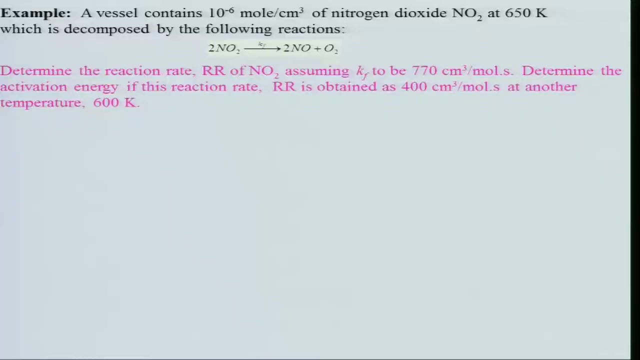 you call is known as the Arrhenius law right And what we will do. we will take an example today: how to use this Arrhenius law and also whether we can determine the activation energy by conducting experiment or not. that we will illustrate through this example. 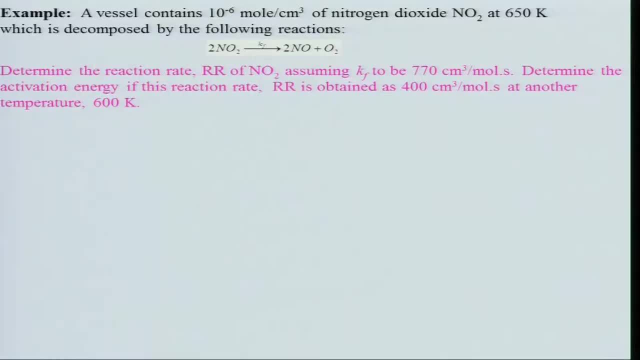 And this example is basically a vessel, you know, which contains 10 power to minus 6 mole per centimeter. So this is a vessel which contains 10 power to minus 6 mole per centimeter cube of nitrogen dioxide at 650 Kelvin. right, If you look at it is basically isothermal reaction which. 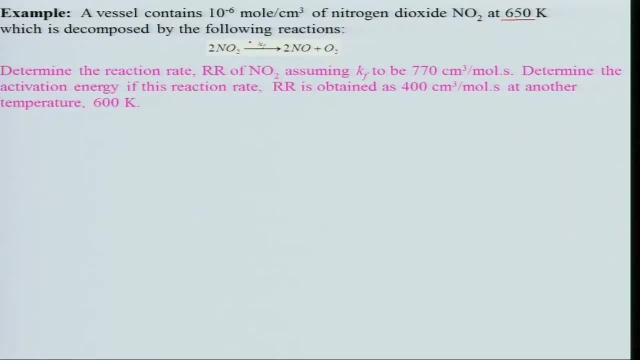 is decomposing to the following reaction, that is 2 n o, 2 goes to 2 n o plus o 2. keep in mind that this is in one direction. the reaction can also come in the backward direction as well. this is a forward direction, backward direction, But we are considering at this. 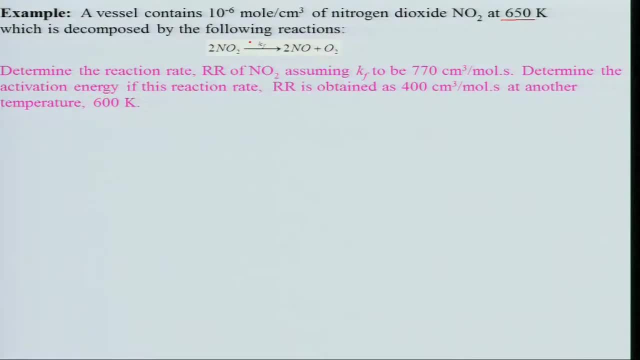 moment only the forward direction. we need to determine the reaction rate of n o 2, assuming k f to be 770 centimeter cube per mole second, And we need to also determine the activation energy if this reaction rate is obtained as the 400 centimeter mole per second. at another 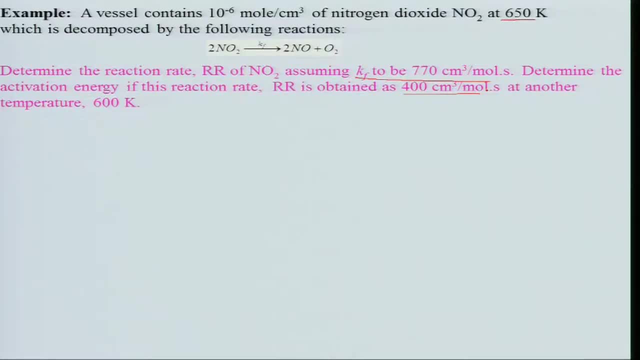 temperature, that is, 600 Kelvin, right? So these are two parts. one is that we need to determine the reaction rate of n o 2 where k f is given. if k f is given, then is it possible? we can find it out right. We will have to. basically. 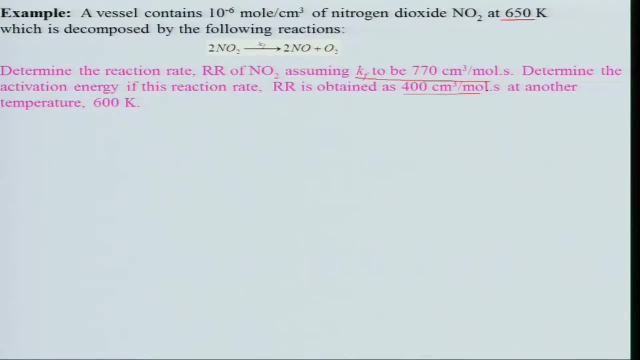 apply the law of mass action- k, f is known to it, known to you- and then we can determine what is the reaction. let us do that. that is a simple part and of course, here we are assuming the reaction to be. What is the meaning of elemental reaction? that we will try to discuss may be after this. 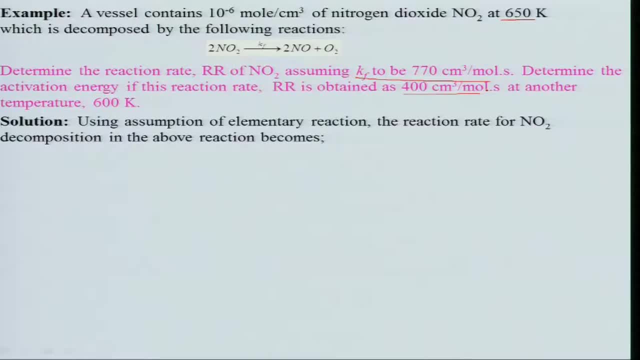 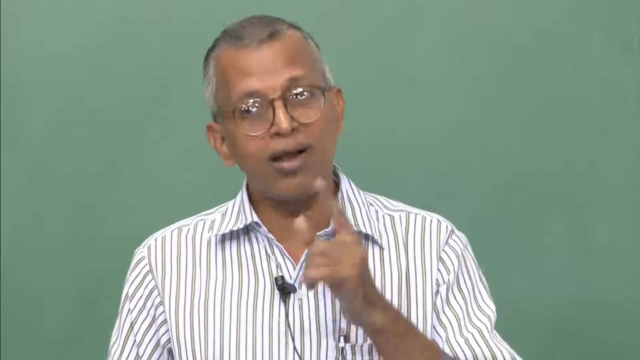 example. but keep in mind that the law of what you call arenas- sorry, the arenas- form of equation is valid only for the elemental reaction, But however we will be using for the global reaction as well, and law of mass action, also right, is also valid for the elementary. 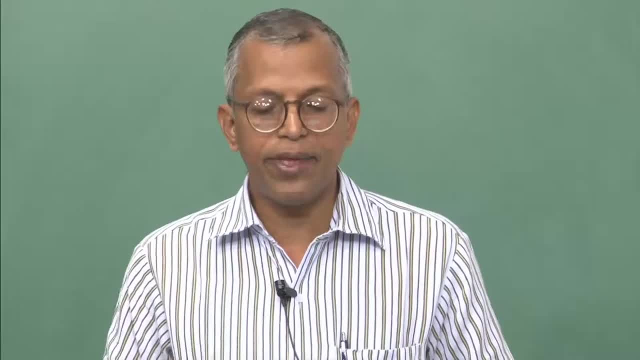 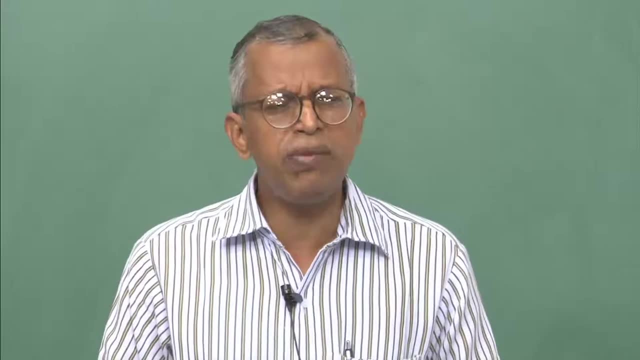 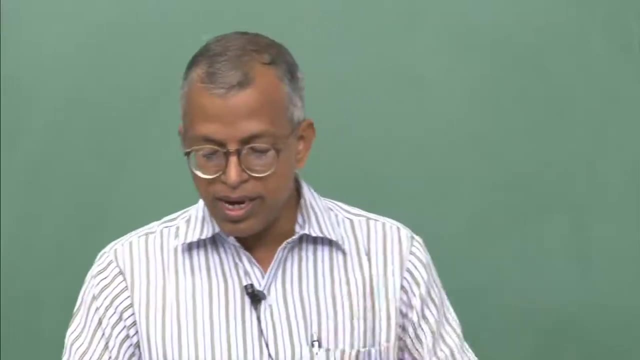 reaction, reaction only. So therefore, whenever we are applying the law of mass action, we should keep in mind that reaction must be elementary. but you must know what is elementary reaction and how it is different from the other reaction, and how many kinds of elementary reaction. 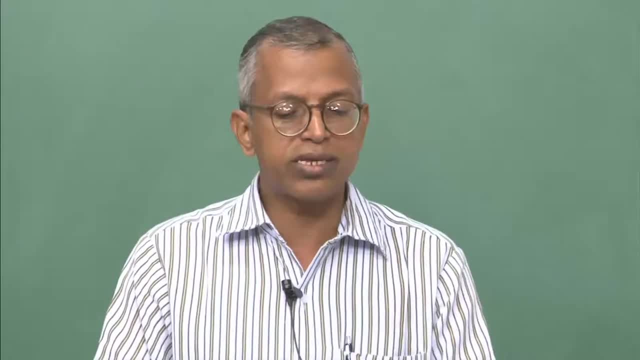 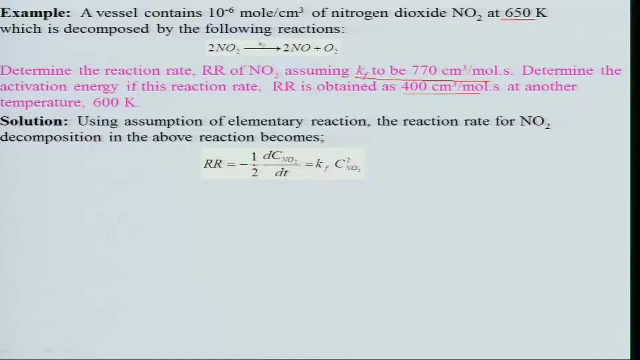 one can think of those thing. we will learn, but before that let us look at this problem. So reaction rate is equal to minus half d c, n o 2 divided by d c. what is it saying? this is a rate of concentration of n? o 2 with respect to, you know, time, of course. rate when I saying: 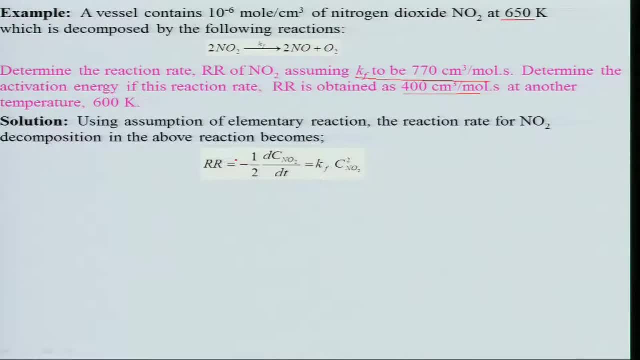 it is means it is time and of course the minus sign is there because it is being decomposed. therefore it is minus and half. of course I have taken because 2, n o, 2 is participating here, So which is equal to k, f, that is reaction coefficient, reaction rate coefficient, and. 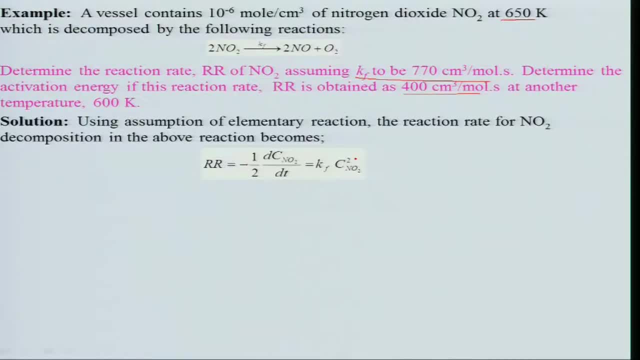 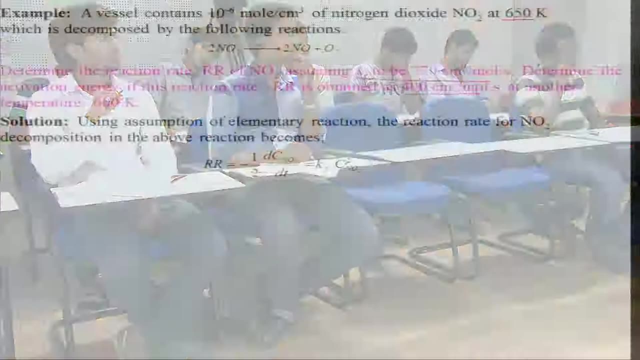 c n o 2 square. why this square comes into picture? because the coefficient in this reaction is 2 and it is an elementary reaction. So that is 2 chromatic coefficient. So therefore it comes as a square. and then what we will do? we, because concentration is given this. 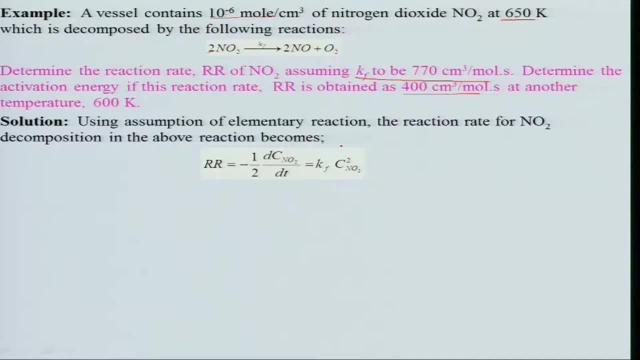 is your concentration of n o 2, and this is known, This is known. you just substitute those values and get the answer, which is very simple, that is acts. you know, 650 Kelvin, that is reaction rate, is equal to minus half d, c, n o 2 by d. 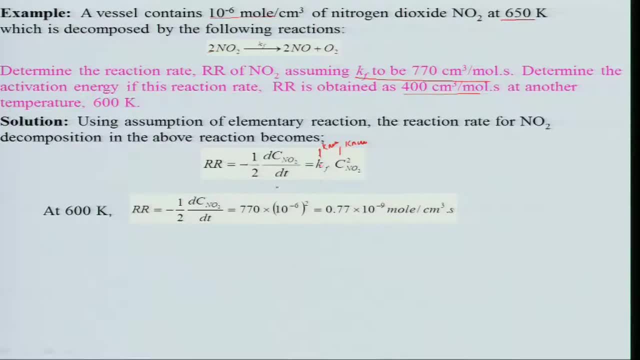 t and you just substitute these values for k, f from here, and then c, n, o, 2 square, you will get this value 0.77 into 10.. So this is the reaction from this one to this. So what we will do, we will write this: 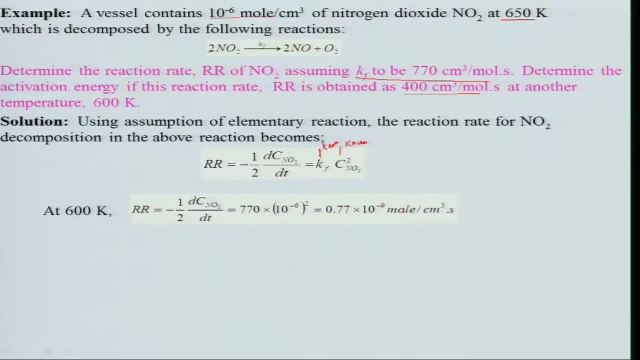 into 10 power minus 9 mole per centimeter. it is a very, very small quantities if you look at, And activation energy for this reaction can be estimated by knowing this specific reaction rate or the reaction rate coefficient. you know both are same at two different temperature. 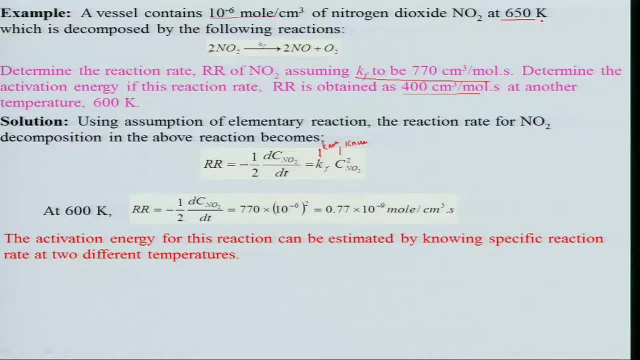 So one is 650, other is of course the 600 Kelvin. So we must know those values. and k f is known, So we can determine that is at t 1 it will be l n. k 1 is equal to l n. 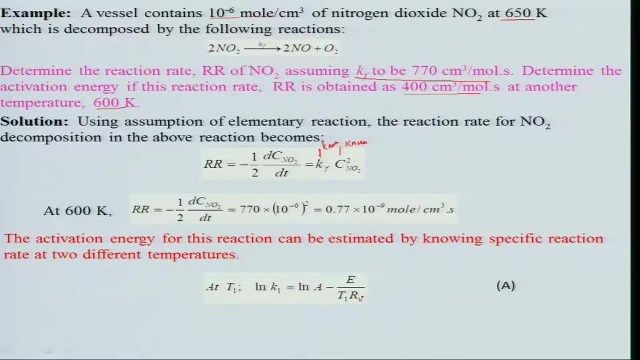 a minus e by t 1. r? u How it is coming, because we know that k 1 is equal to a e by r t 1. of course this is r? u. So if I take both the side, log the natural gate l? l n, k 1.. 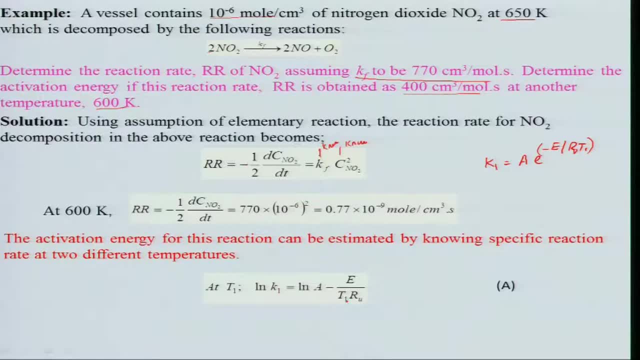 So l n k 1 is equal to l n a minus e by t 1 r? u. Similarly I will do for the at the temperature t 2, that is, l n k 2 is equal to l n a minus e by t 2 r? u r? u is the universal. 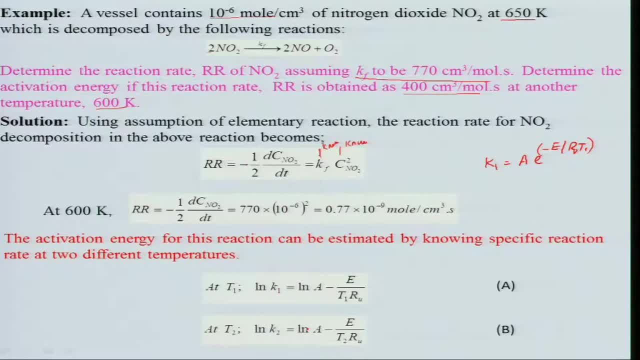 gas constant. What I will do? I will just say: like equation 1 minus equation, like equation a minus equation b will give what if I just say this is minus And it cancel it out, what will happen? So this become minus, this become minus, this become. 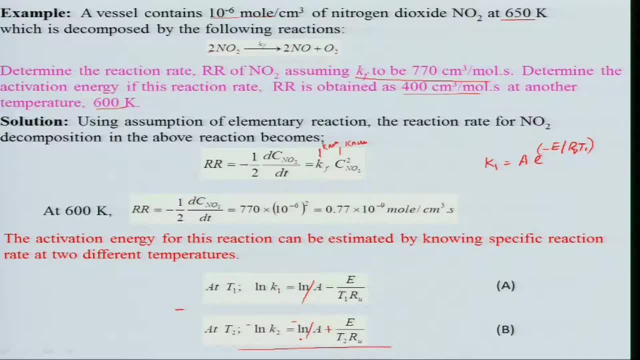 plus. So this will cancel it out what I will get. I will get l n k 1 minus l n k 2 is equal to e by r t 2 minus e by t 1 r? u. I can get that and we will simplify this and get those.